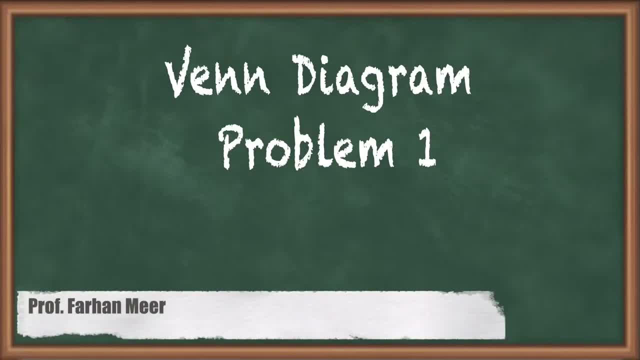 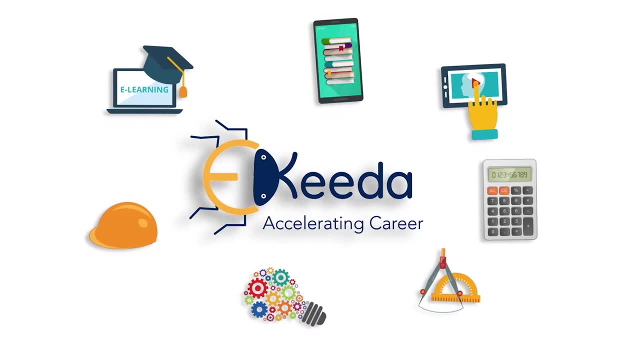 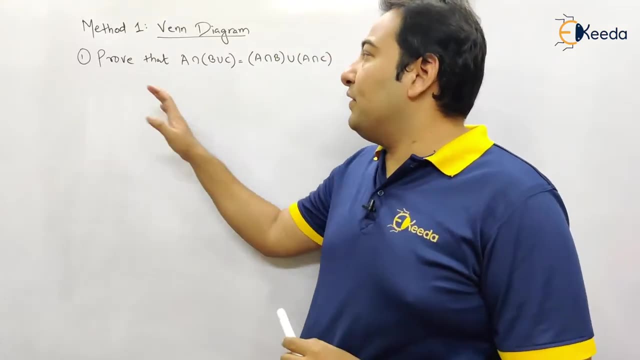 Hello friends, in this video we will be discussing Venn diagram, problem number 1.. Welcome back, friends. Now we will be discussing Venn diagram, problem number 1.. Here we need to prove this particular problem- LHS equal to RHS, and we will be using the first method. 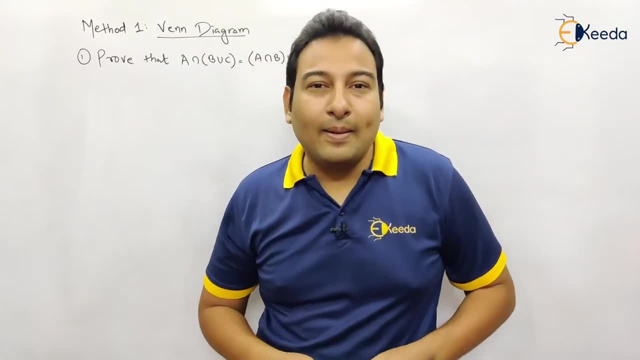 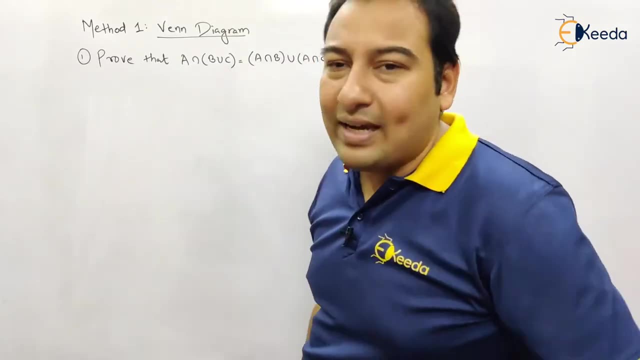 for proving it, that is Venn diagram. There are actually two methods. There is one more method that we will be discussing later on. First of all, in this video, we will be discussing this problem by using Venn diagram. So this is a very popular method that we have learned till childhood. 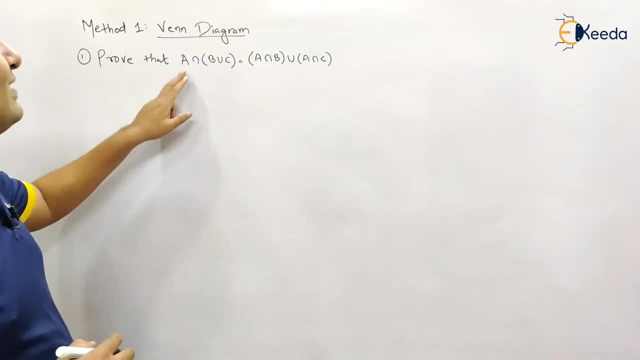 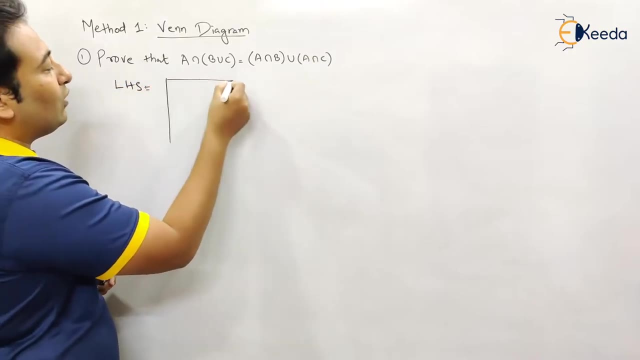 So let's do it quickly. First of all, there are three sets: A, B and C. Therefore, first of all, let us prove LHS. There are three sets. Therefore, in all the boxes of Venn diagram, I will be. 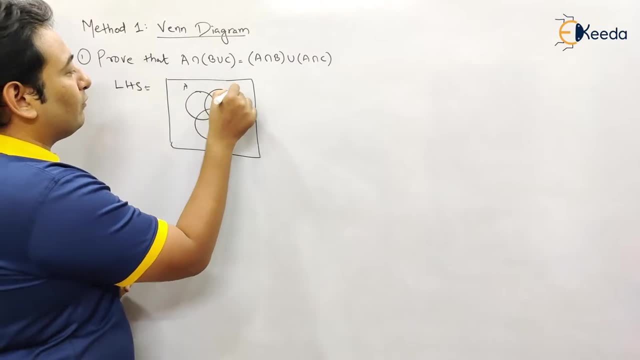 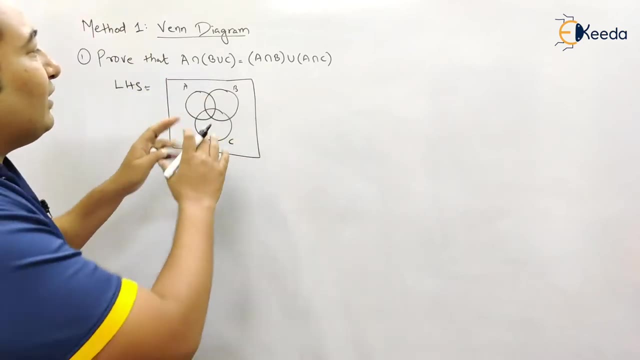 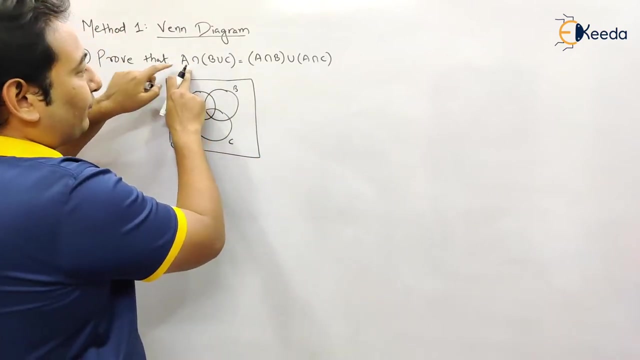 having three sets: A, B, C. So see the way I am solving the problem. First of all for LHS. let us break this problem. LHS. Let us consider LHS first and in LHS also, let us break the problem. Here. there is one A, The one element is A, So let's shade A. 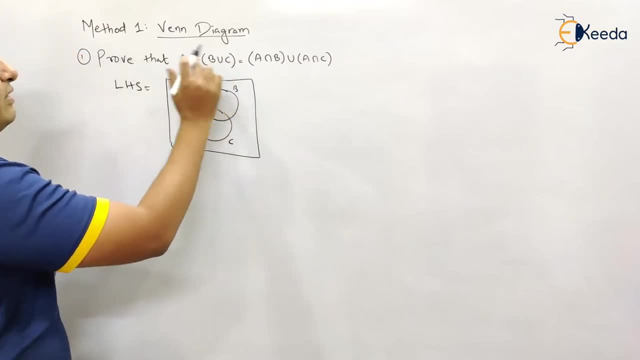 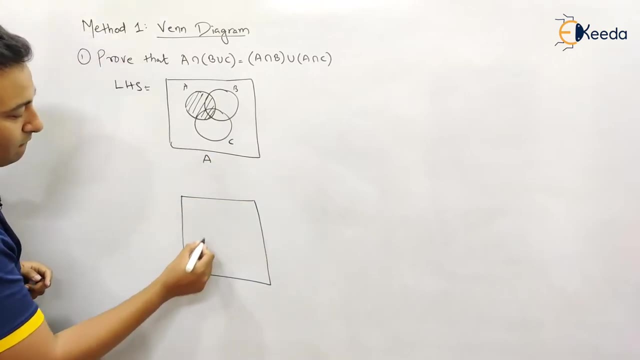 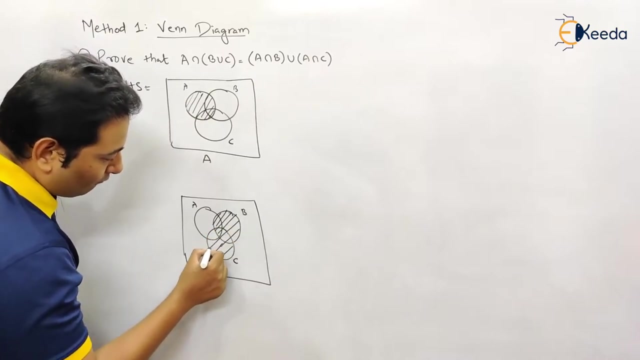 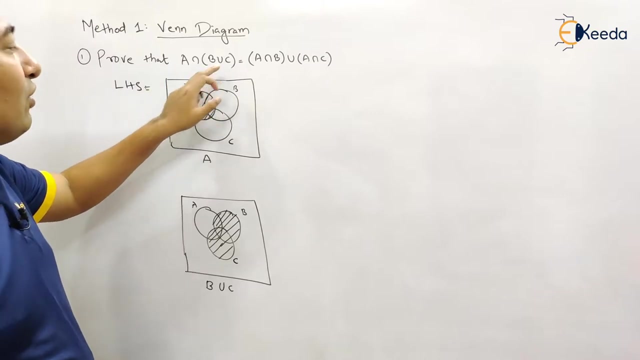 So this is my A. Now let us shade B union C. So this is basically A. Now B union C. That means all the elements of B and C. This is my B union C. What is next? I want intersection of both. See, I am ready with these two. 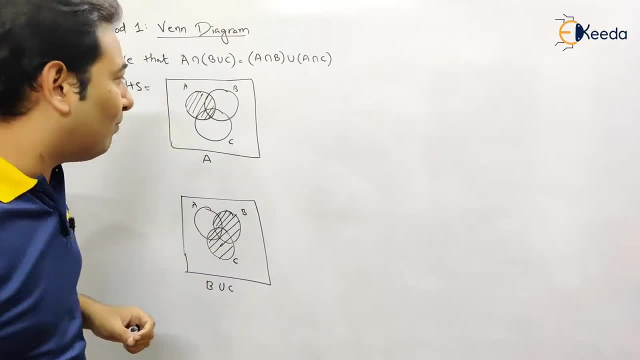 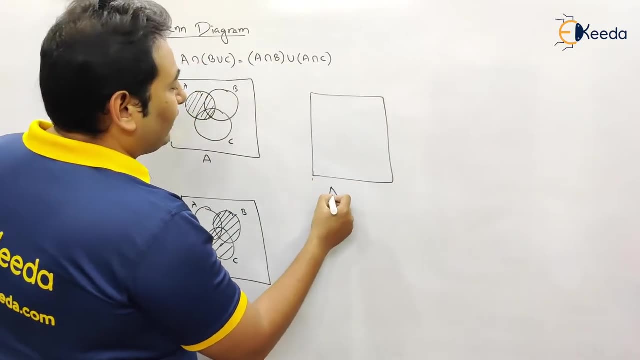 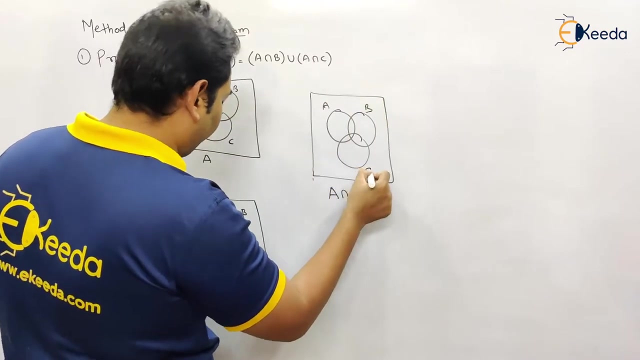 Now let us find it out: the intersection. Intersection means common. So what is common in these two diagrams? So that we are going to divide and my LHS will be ready, That is LHS. So we have A intersection B, union C. So let us see what is common between these two diagrams. 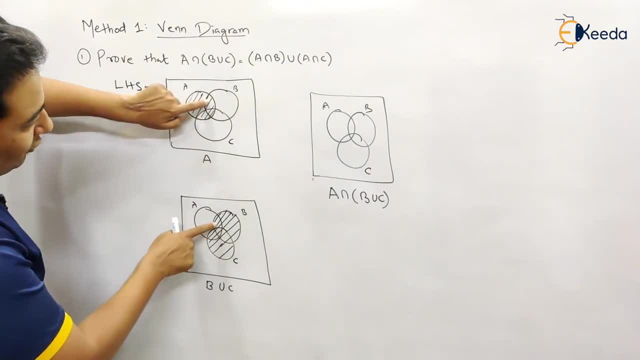 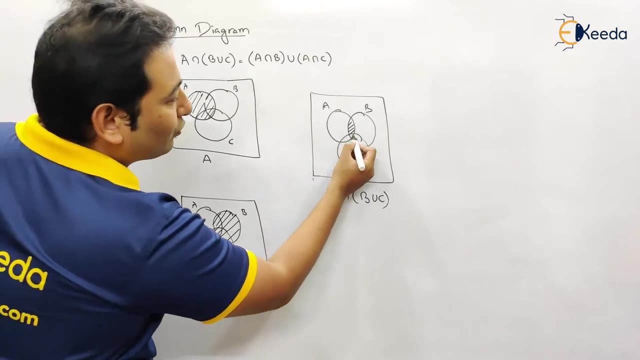 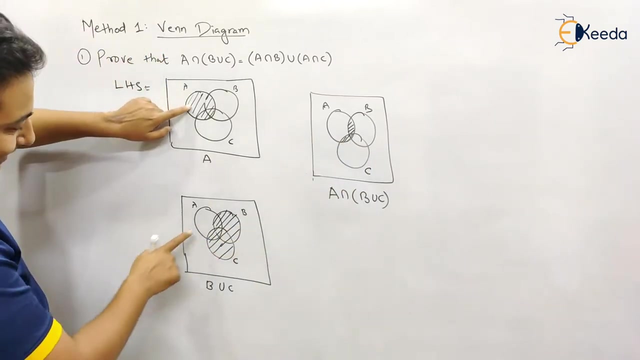 See here: This part. This part is common, So that will come here. What else? This intersection, This is also common, So this will be shaded. This part is also common, So this will be shaded. What else? This part is here but not shaded here, So we are going to leave it. 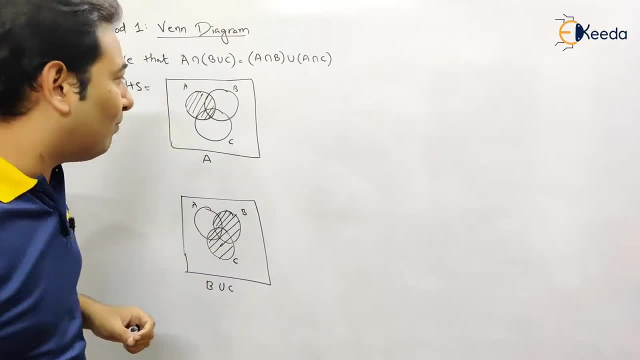 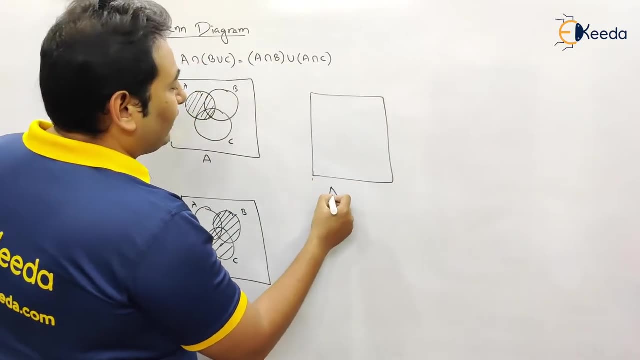 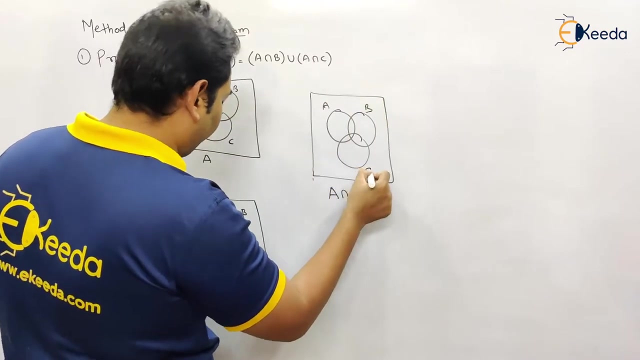 Now let us find it out: the intersection. Intersection means common. So what is common in these two diagrams? So that we are going to divide and my LHS will be ready. That is LHS. So this is A intersection B, union C. So let us see what is common between these two diagrams. 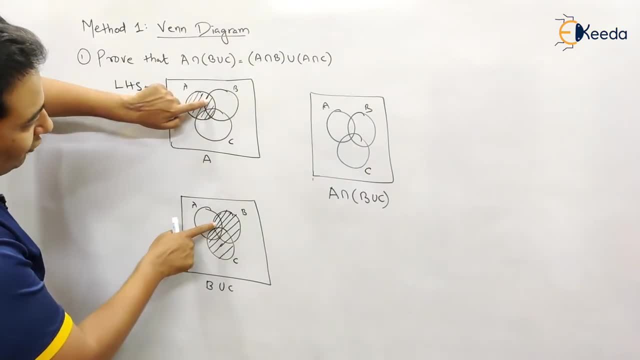 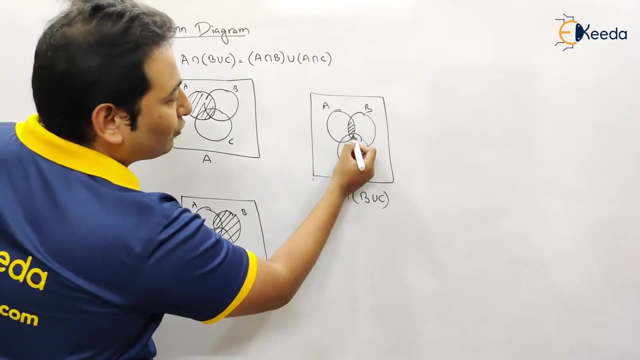 See here this part. This part is common, So that will come here. What else? See here this intersection. This is also common, So this will be shaded. This part is also common, So this will be shaded. What else? 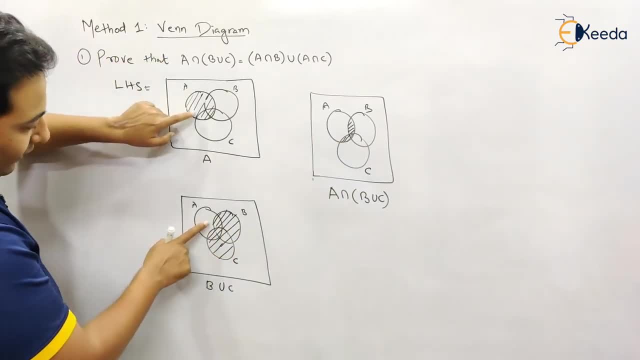 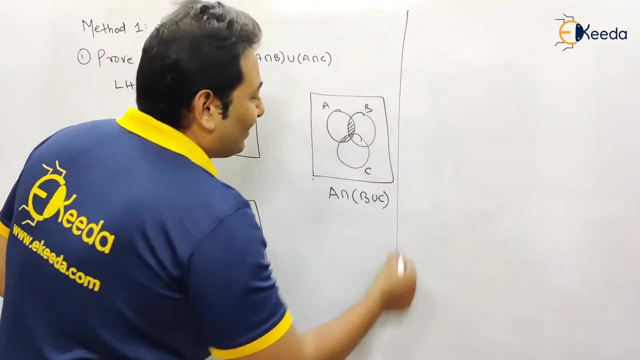 This part is here, but not shaded here, So we are going to leave it. This is going to leave it. This is going to leave it. this is going to leave it. so this is your result. a, intersection b, union c. now we're going to write. 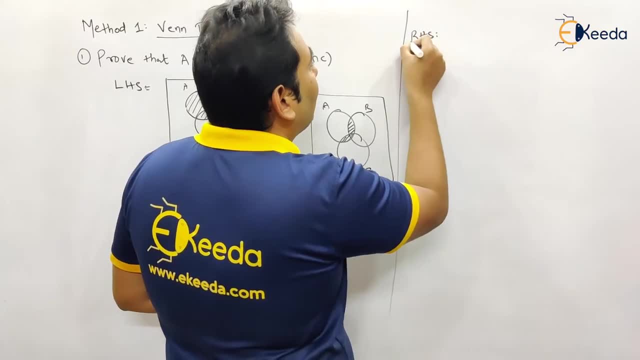 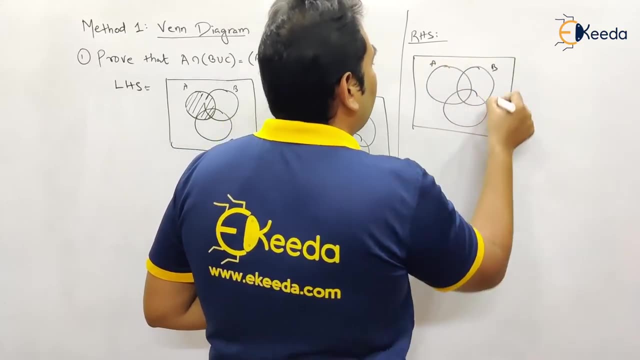 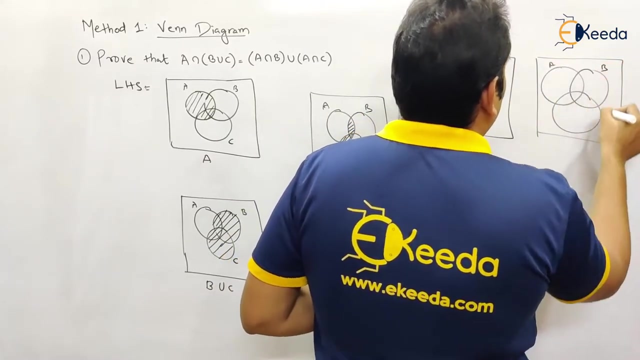 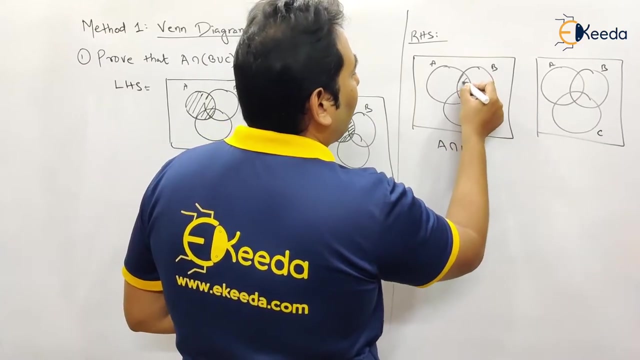 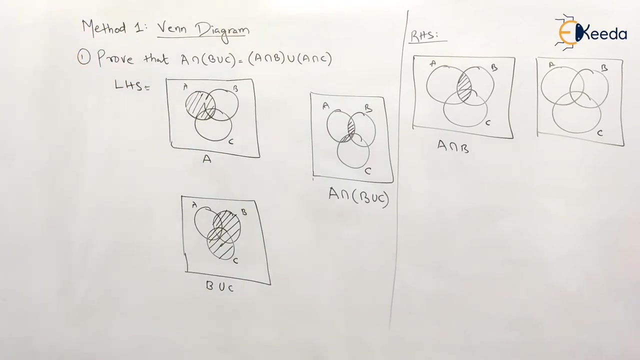 it down rhs in rhs. if i'll break down rhs into two, this is a b, c, a b c. the first bracket is a intersection b. so what do you mean by a intersection b? common between a and b? so this is your a intersection b. so while shading a intersection b, forget about the third part, that is c. 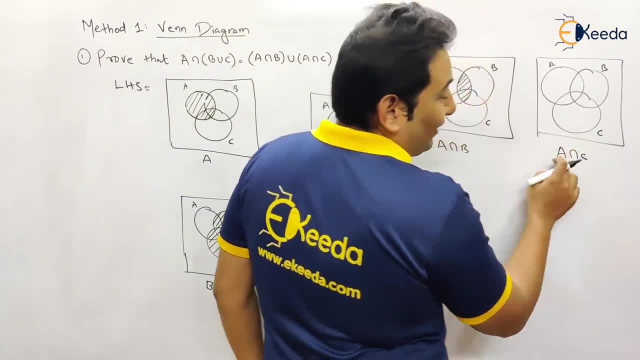 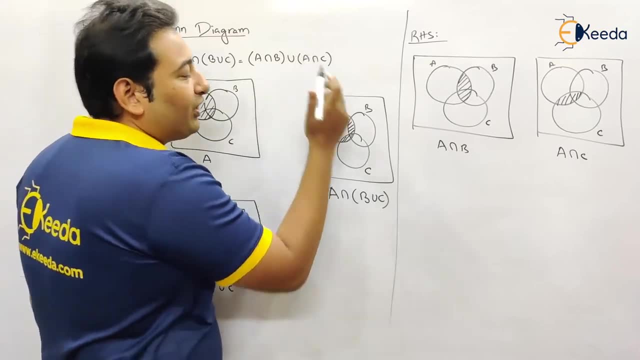 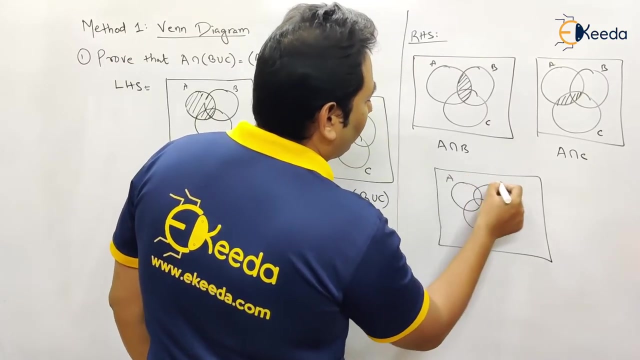 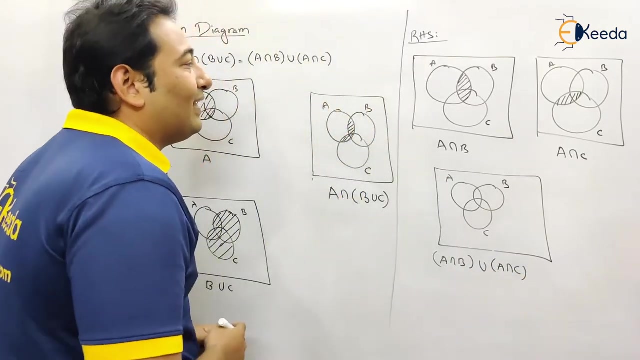 a intersection c. so concentrate on a and c, only forget about b. so this is your: a intersection c. what is next? i want to find union of both. union means the total shaded area. i want a intersection b, b union, a intersection c, so total shaded area. so say this: this is this shade. 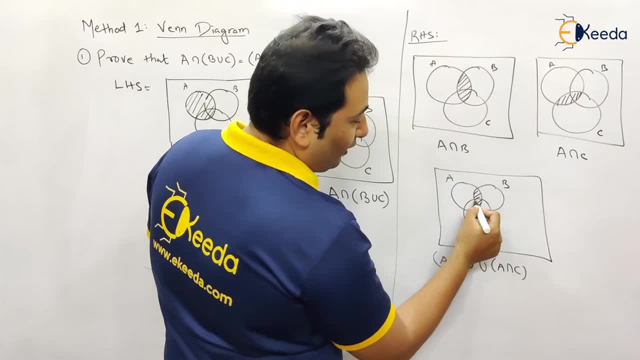 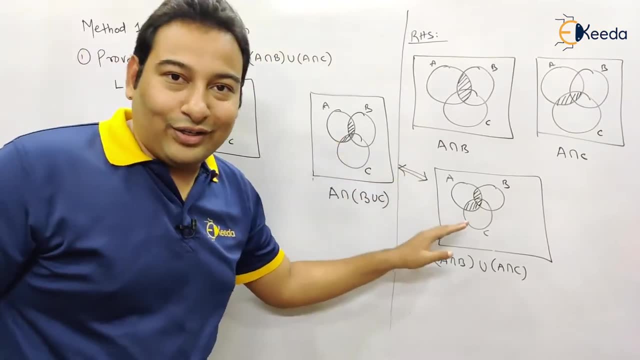 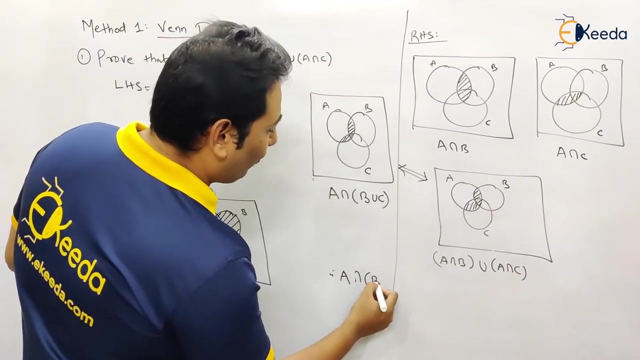 as well as this shade, this one and common part you're going to consider once now. check this: see, both the diagrams are equivalent. so that means we are done with the proof: lhs equal to rhs. so this is the equivalence we proved by using venn diagram. i hope this is clear in the next. 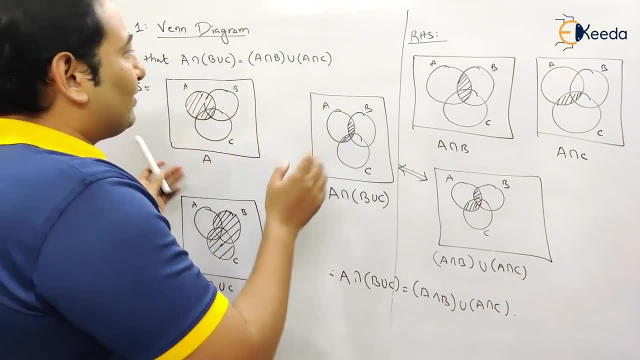 video. we'll be discussing two more examples on venn diagram. thank you,